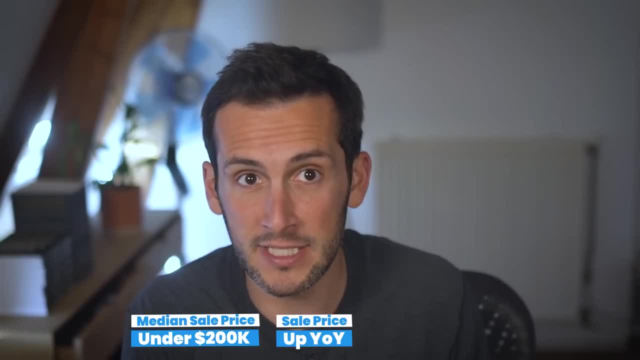 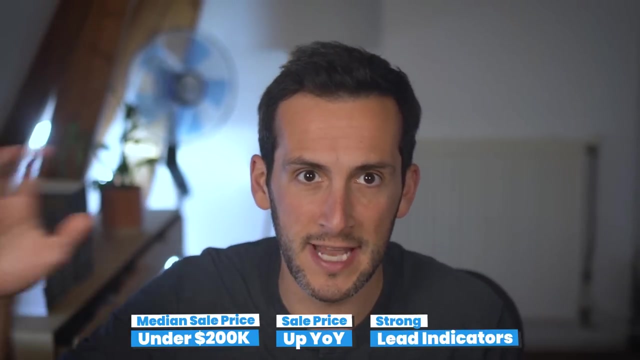 correction and some markets are declining and have over the last year, while other markets have stayed pretty stable Or strong, And I only picked markets that have seen positive home price appreciation over the last year. And then, third, I looked at some lead indicators for what might happen over the next. 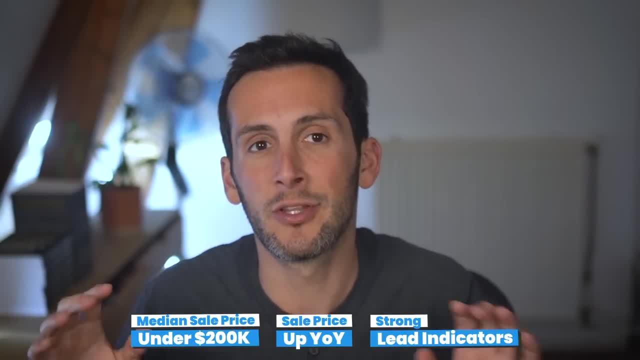 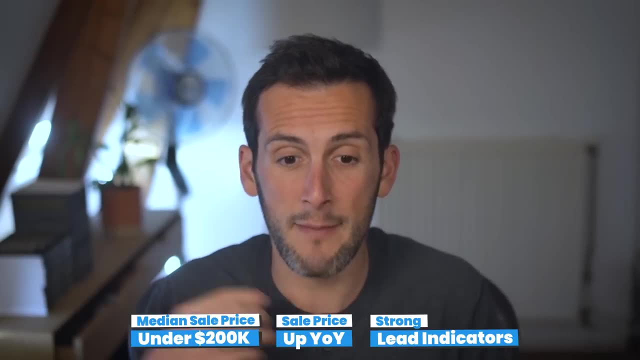 couple of months. Of course, we obviously don't know exactly what's going to happen, but you can look at some measurements of supply and demand, like inventory levels, new listing and days on market, And so I picked ones that I- this is subjective but I believe, point to a pretty 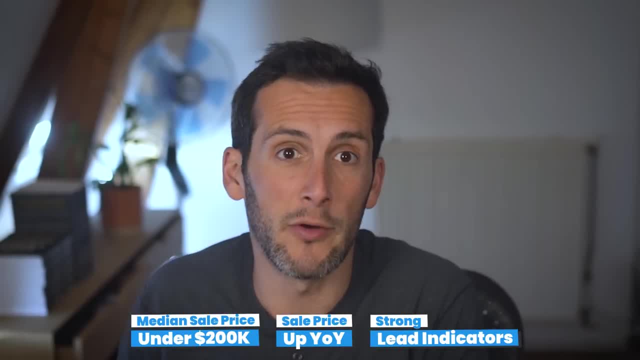 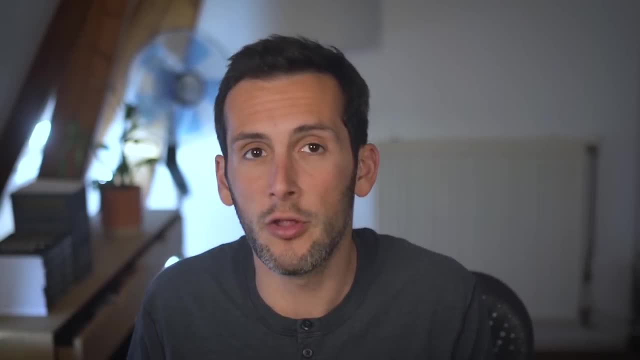 competitive marketplace for the summer, where prices might keep up, And I also looked at some of the things that are going to keep going up. And then, lastly, I also looked at population growth, rent and some cashflow potential. So I looked at all these different variables before we get. 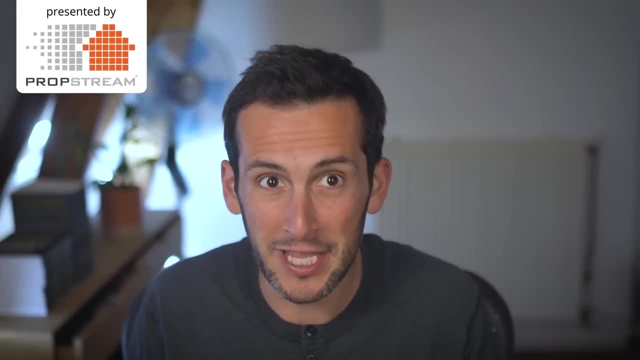 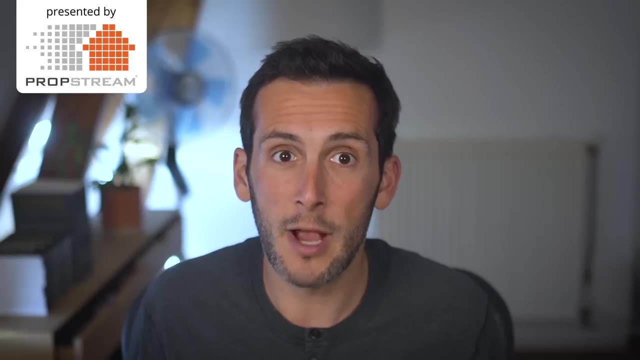 into these five markets. You all know how much I absolutely love data, but to get good deals, there's really only one data source you need, And that's PropStream. PropStream helps investors find motivated sellers in any market across the U? S, with hundreds of different filters you can use. 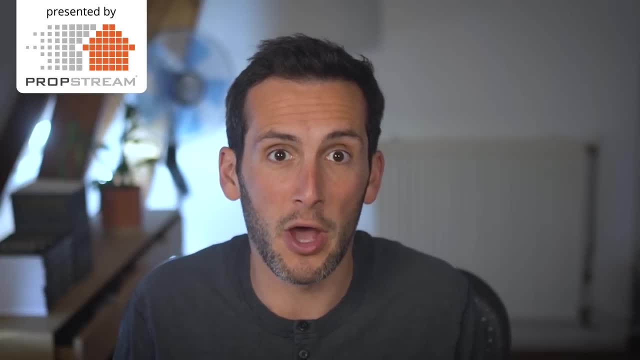 to find the perfect deals for you. You can search both on and off the website and you can find all market for properties. You can run comps, get in touch with sellers using these built in marketing tools that are super easy to use, And you can analyze deals to your heart's desire When inventory. 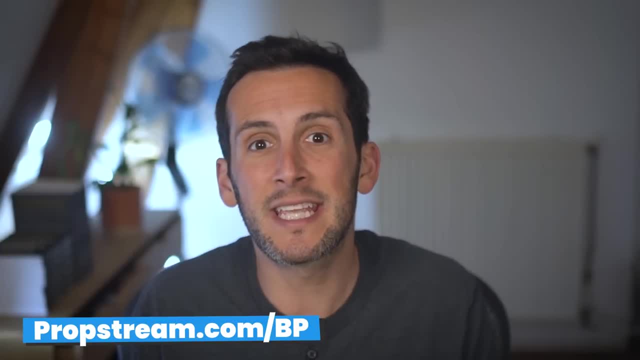 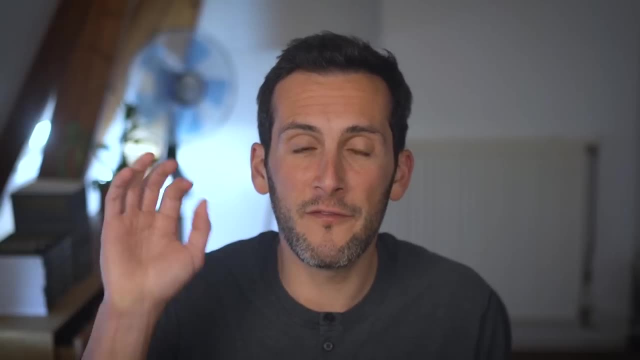 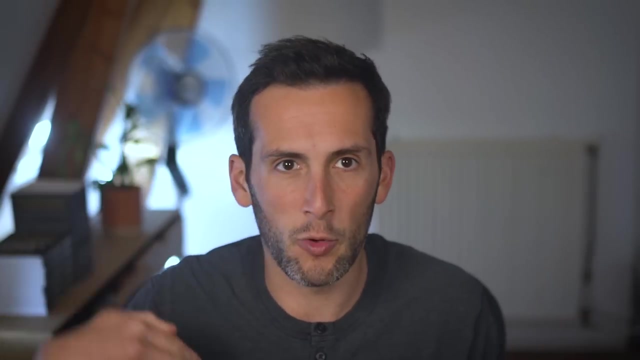 is tough to come by like it is right now. PropStream is the key to finding your next deal. Check them out at PropStreamcom. slash BP Now for our five great markets where the median sales price is under $200,000,. I'm just going to go in descending order, So the first one's going to be: 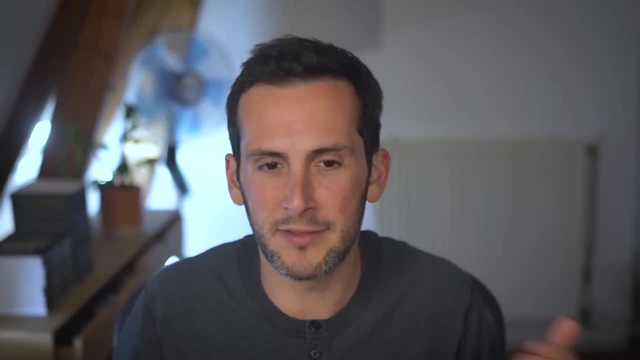 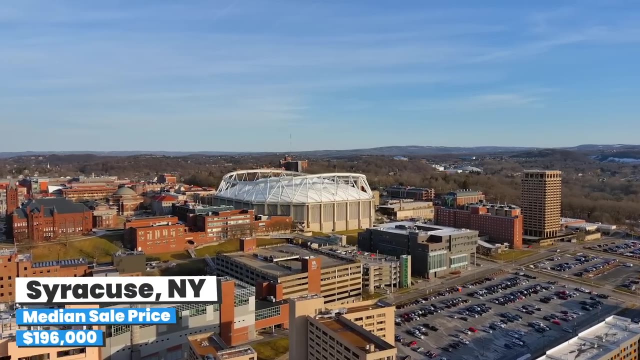 the most expensive and go down to the least expensive, but they're not ranked in any particular order. For our first list it is Syracuse And, like I said, that's the most expensive city on the list, with a median sales price of $196,000.. So, again, most expensive on. 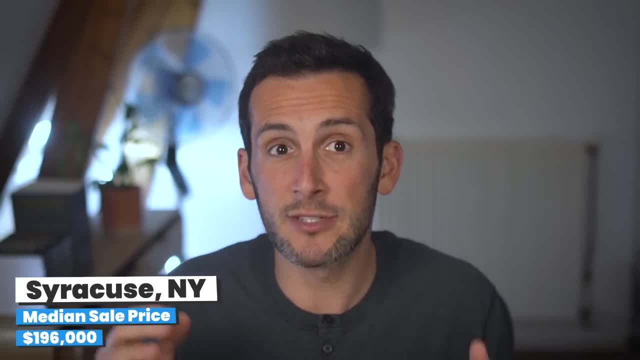 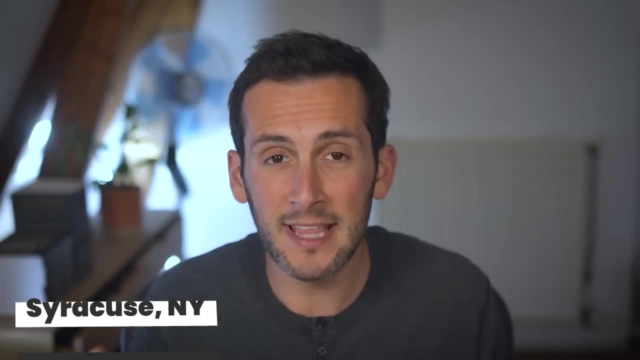 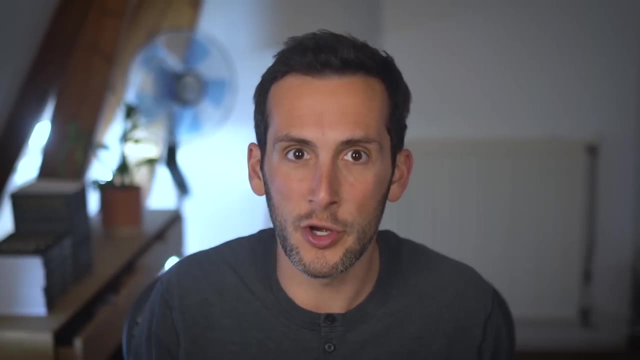 this list, but about half the national average. Syracuse is really interesting because it remains very competitive. It's actually one of the more competitive markets in the entire country. I'm saying that because there's this really interesting metric called the sale to list ratio And that basically measures how much over or under the listing price property. 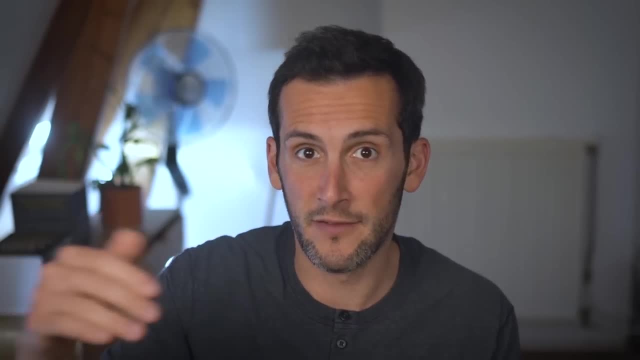 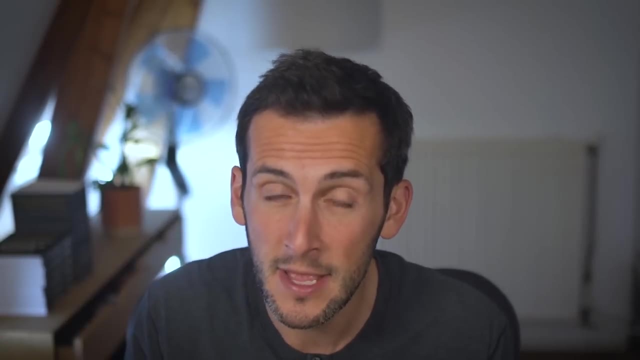 sell for And Syracuse is still over a hundred. The vast majority of markets in the country right now are under a hundred, meaning that people are bidding under asking price, But in Syracuse it is still a strong seller's market where the sale to list ratio is over a hundred percent. 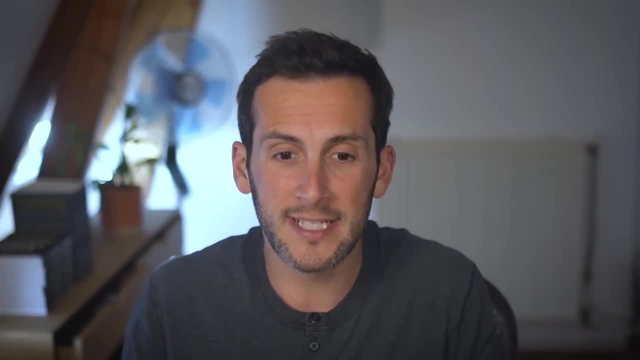 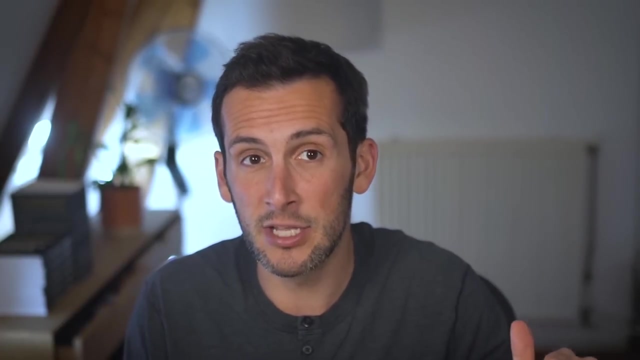 So this is one of the reasons. remember I said that my criteria were that I saw lead indicators up. This is a strong lead indicator that it's going to be a competitive market over the summer. We're also seeing days on market which are rising nationally- declining in Syracuse, And so 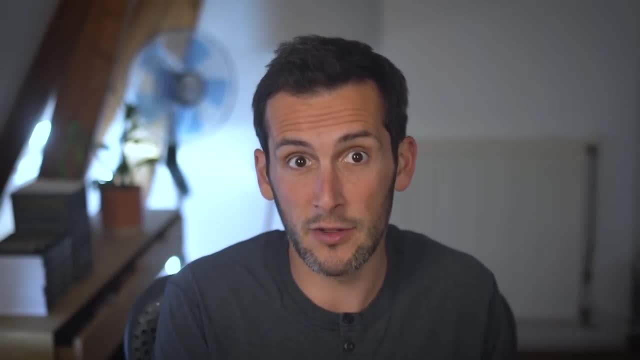 it points to a really good market that is relatively affordable- Just over the last year, prices have gone up 11%- and it has a really strong cashflow potential. When I say cashflow potential, I use this sort of rough metric called the rent to price ratio. 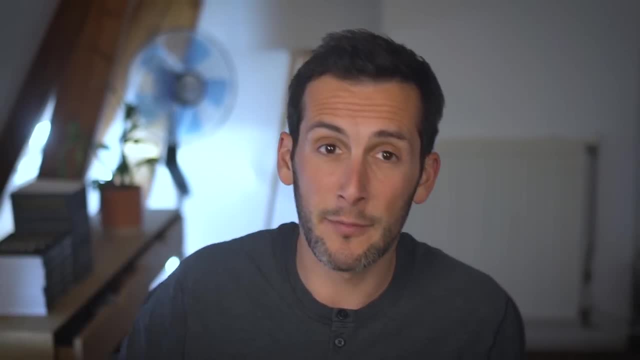 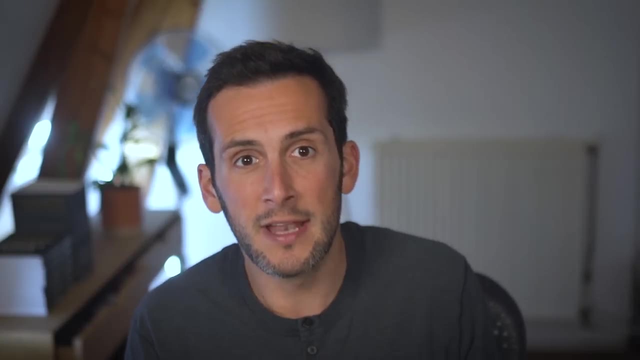 which basically just combines the median rent in the area To the median sale price in the area And it gives you a rough idea of if there are going to be good deals in that area that offer strong cashflow. And generally speaking, I like to think that if a rent, like a whole area has a rent to price ratio of like 0.65 or above, you're going to be able to find cashflowing deals there. If it's below, it's still possible to find cashflowing deals. It's. just going to be harder, And so when I look at Syracuse, I see a market that's affordable, growing quickly and has really good cashflow potential. The second city on our list is Lansing, Michigan, with a median sale price of $191,000.. And again, 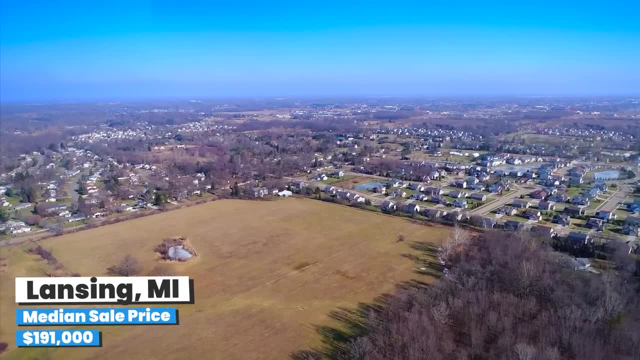 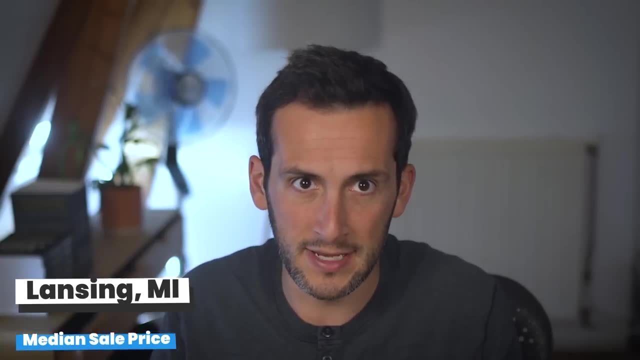 prices are still rising here, but at a more reasonable rate. In Syracuse prices were going up 11% year over year, as you remember, which is well above normal, And in Lansing they're at 6.3%, which is still above normal, but it's getting to within the realm. 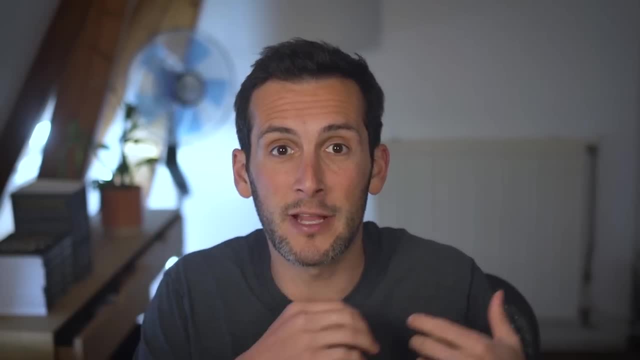 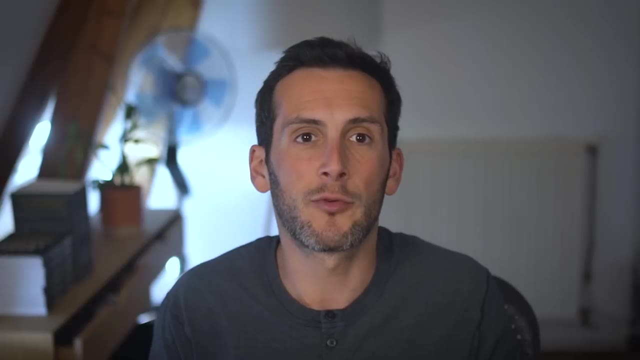 of reason And personally, that's what I would like to see- is the housing market return to a time where prices are going to be more reasonable, And I think that's a good thing. Prices go up 3% or 4%, or about the pace of inflation, And so that's what we're seeing. 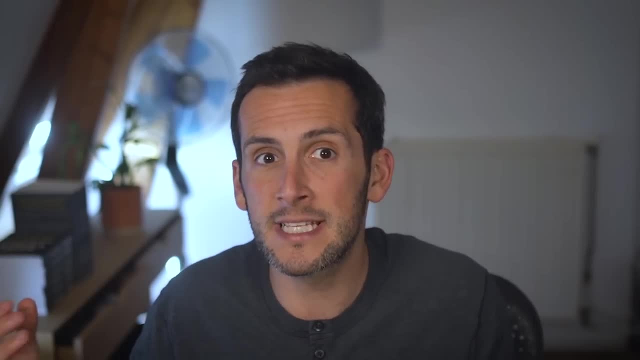 in Lansing, which to me points to a pretty stable housing market. The thing that really stands out to me about Lansing is that inventory- the amount of homes that are for sale- is absolutely in the basement. It's been going down over the last year, But when? I compared inventory right now to the same time period back in 2019, just to get a sense of how of the pandemic. right now, there is only 44% of the inventory as there was back in 2019.. So there is basically nothing for sale in this entire city, which has contributed to prices continuing to go. up. Another thing I really like about Lansing is that population growth is pretty strong at 0.6% per year, And there is a solid cashflow potential with a rent to price ratio of 0.73%. For our third market on the list, we have Scranton. 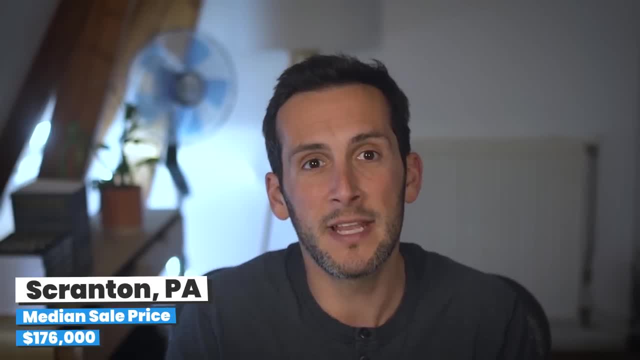 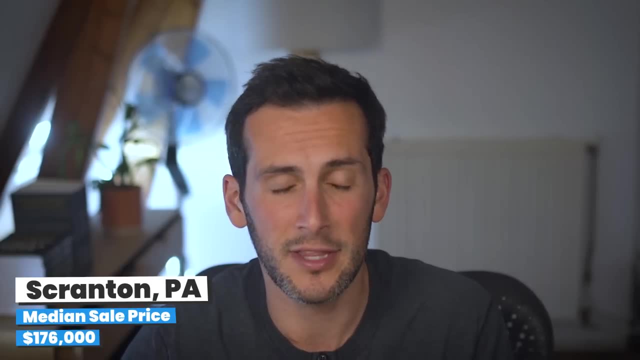 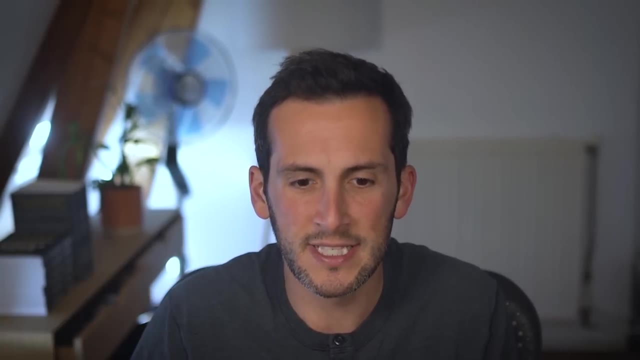 Pennsylvania, of course, the home of the famous Dunder Mifflin, with a median sale price that drops down a little but pretty considerably to $176,000.. And this crazy thing about Scranton is that inventory, which has been low sort of throughout the pandemic in all sorts of markets, has dropped. basically off a cliff this year. It's fallen 45% this year alone And if you've been following the housing market on a national level, you would expect inventory to be down by 0.6% per year. That's going to be going up, at least on a national level, this year when interest rates are going up. 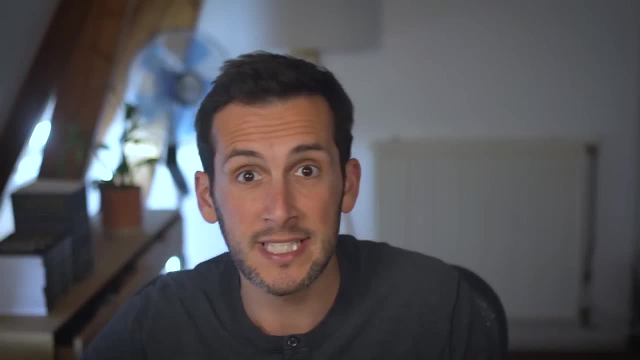 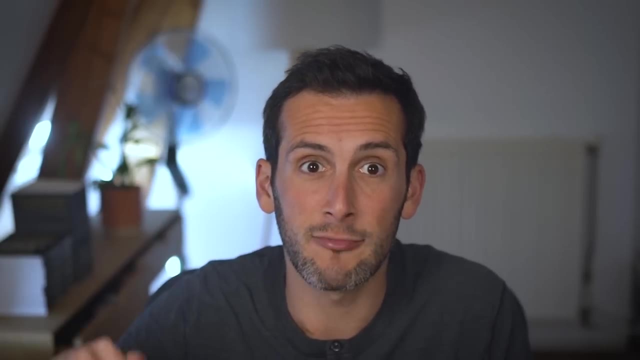 That pulls demand out of the market. That means that more homes are usually sitting on the market and that pushes inventory up. But inventory is falling pretty dramatically in Scranton right now, which means that there is likely going to be a very competitive buying season over the summer. 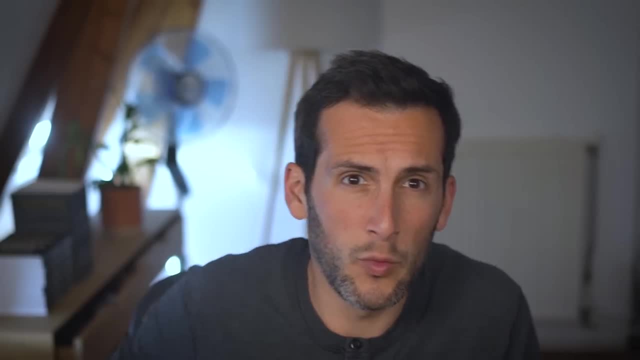 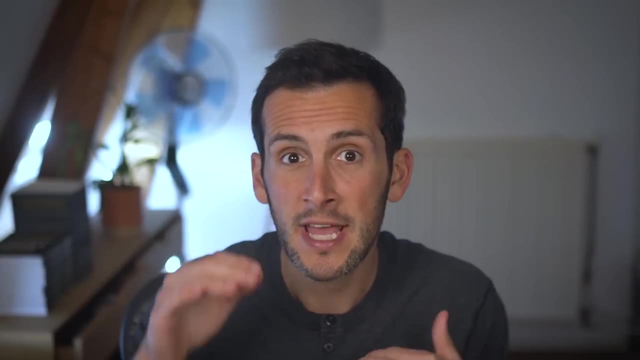 here in Scranton. One of the things that's going on in Scranton that's kind of weird, despite the low inventory, is that the list to sale ratio- remember about that in Syracuse being over 100, is the lowest on our list at 97.5%, Which means that 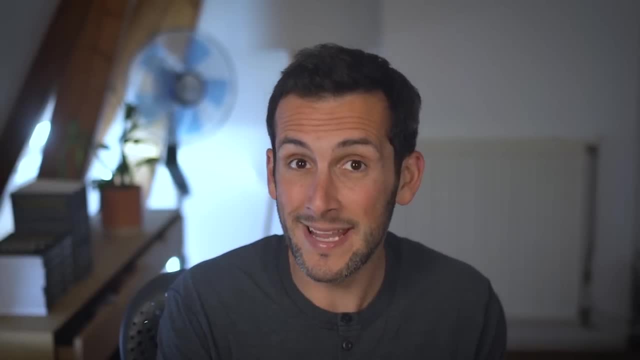 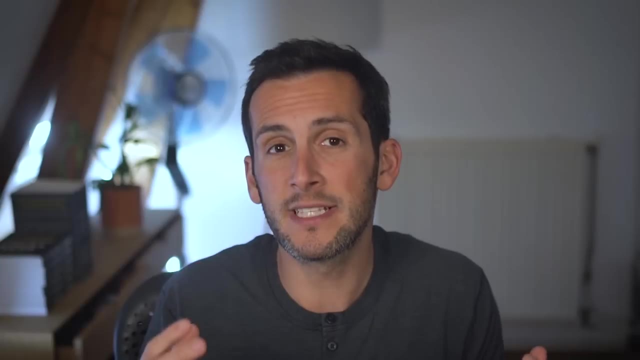 even though there's not a lot of stuff on the market, people are still bidding under asking price and are still able to get it. So I see this happening in a lot of markets where prices are still going up but the list to sale ratio is off, which just means that sellers are probably reaching a little bit with their list price. They want to get their best, obviously, and it's well above where it would have been last year, but it's a little bit too high And so buyers are able to get under list price, but still well above where it was last year. 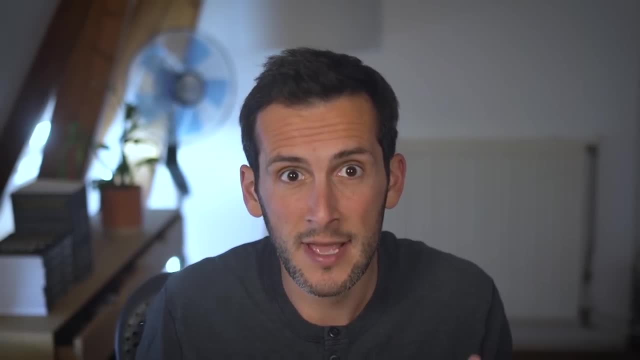 So if you're considering buying in Scranton, just take note of that, because it means that you probably have an opportunity to offer below asking and hopefully negotiate with the seller despite low inventory. For our fourth market on the list, we've got Toledo, Ohio, Median sale. price $173,000. And it has gone up 6.1% over the last year. Just like a lot of our other markets, the lead indicators in Toledo are strong. Inventory and days are. market are shrinking here, which means there could be further price appreciation in Toledo over the coming months. 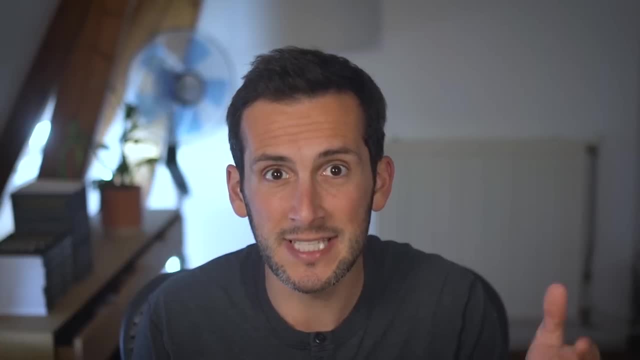 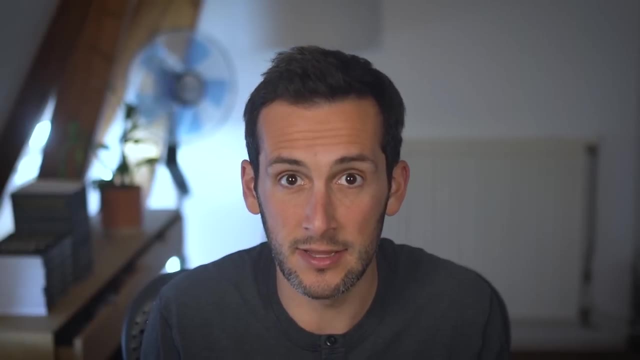 And even days on market. I just said this, but even days on market have fallen over the last year, And that is very different from a lot of markets that we're seeing in the country right now. Days on market is just basically a measurement. How long the average property in the market sits on the market before it is put under contract, And even in markets that are doing well and have price appreciation across the country, days on market has been ticking up as buyers have been a little bit more patient. 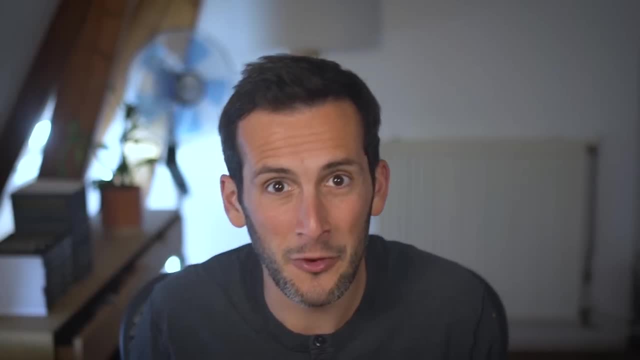 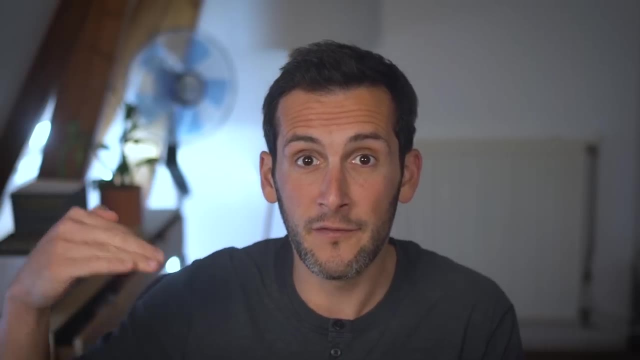 You know they're not submitting blind offers without even seeing it anymore. They're being. you know there is some return to normalcy here, But in Toledo we're actually seeing days on market fall, which is unusual and again suggests a contraction. Market place. The one thing about Toledo you should know, though, is that rent here is only about eight hundred and fifty dollars a month on average, which makes it the worst rent to price ratio on our list of only about point five percent, So that means that cash flow prospects are lower than the other markets on this list Doesn't mean that it's impossible, but it is something to know. But on the flip side, Toledo is really strong population growth, suggesting that demand will continue well into the future. Last but not least, on our list.